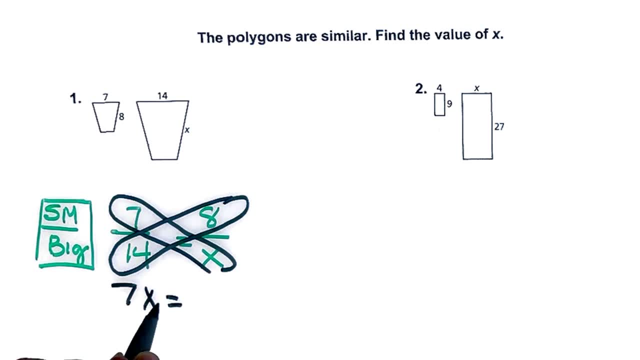 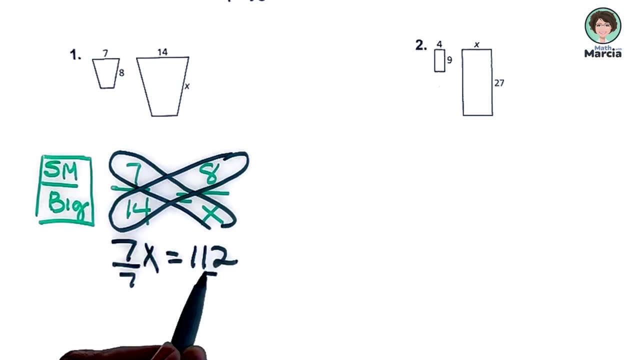 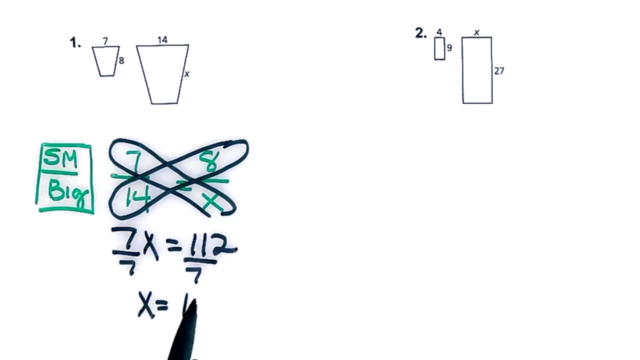 multiply seven times x is seven x, and eight times 14 is 112.. I need to get my variable alone. So the x is going to be equal to 112 divided by seven. So I'm going to multiply seven times x is 16.. Here is our missing side. 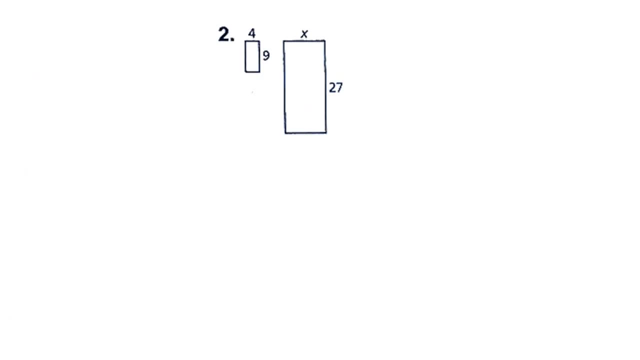 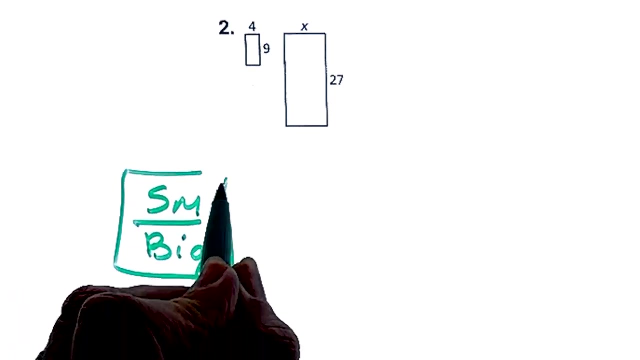 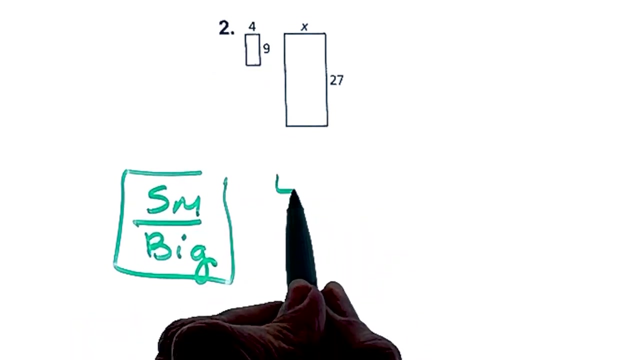 All right. so let's look at number two. Here I have a small rectangle and I have a larger rectangle. So again, I am going to go ahead and I am going to write small over big. And that's my brain getting ready to solve this problem. And now the small base is a four. 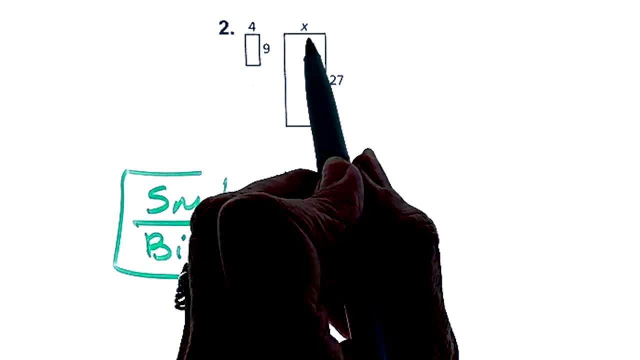 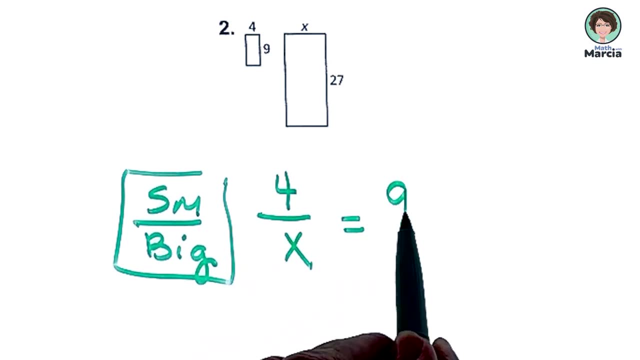 and the large base it corresponds with it is an x Going to the side of the rectangle, the small is a nine, But notice, the large is a 27.. Again, my small values are my numerator, my larger values are my denominator. 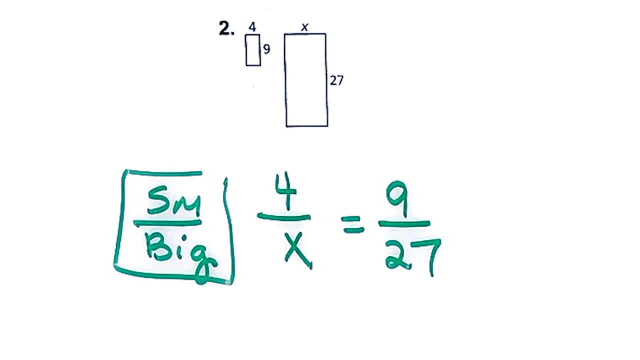 And so now we will do the exact same thing, We're going to go ahead and we will find the cross products. So nine times x is nine x, and four times 27 is 108.. To get the x by itself, I have to divide by nine. 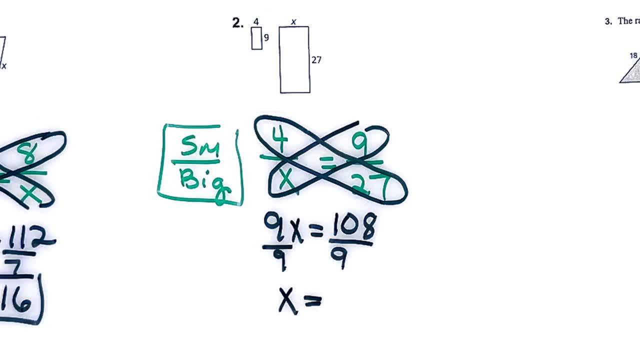 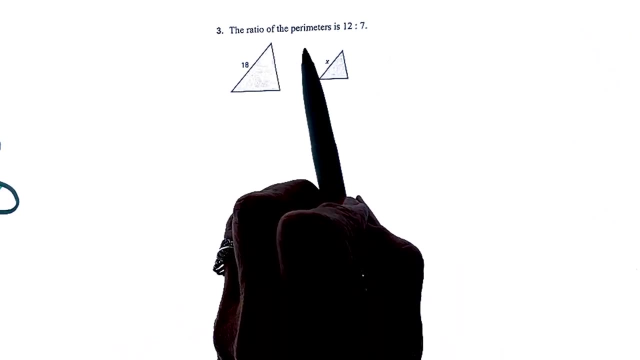 So our base- that actually that is missing- is a 12.. There's our missing part. All right, let's look now at a problem that's a little bit different. It says the Ratio of the perimeters are 12 to seven. 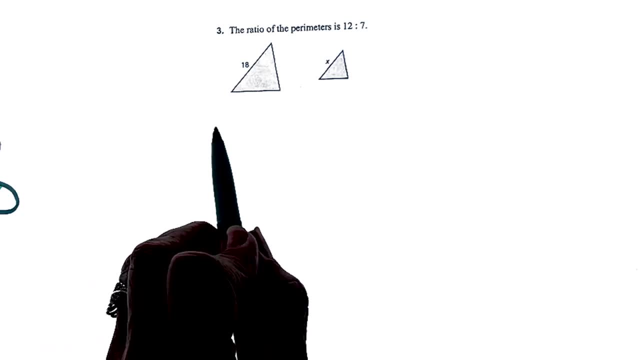 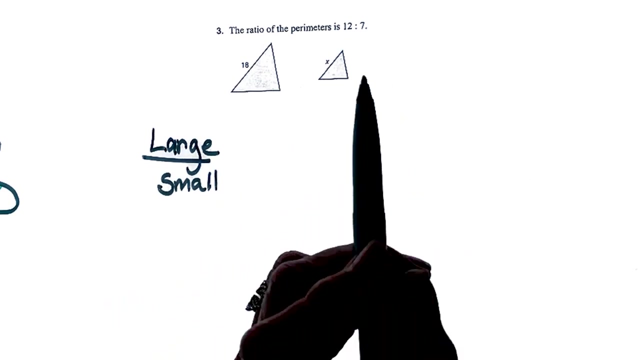 Well, if I know the ratio of perimeters, I again: large triangle, small triangle. So I am going to go large Over small And I know that this has to be my larger one because the perimeter is larger, so it's a 12..